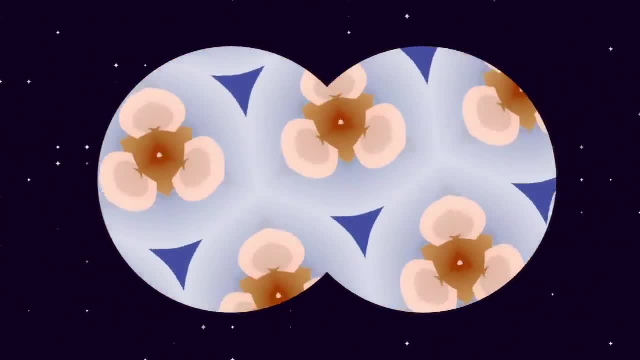 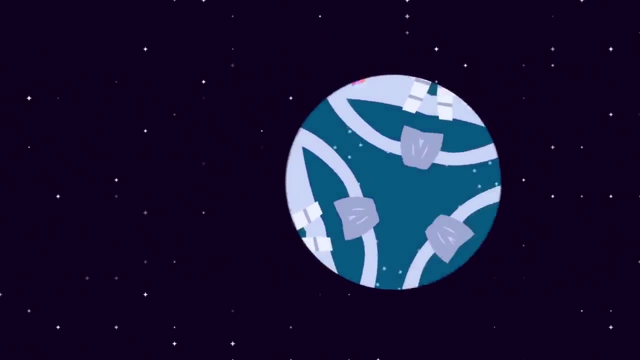 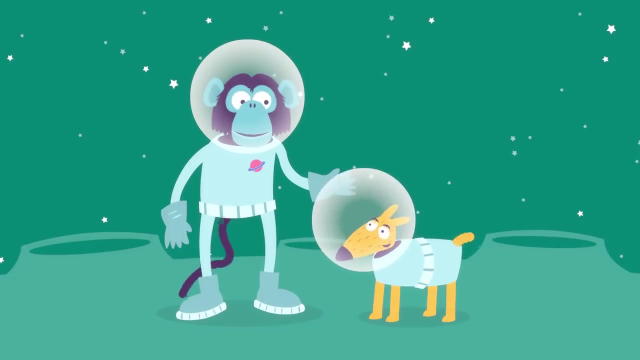 through. Oh look at the colours. They're all spinning around. They're amazing. Oh, look the shapes. Can you see the picture? Yes, look, It's a monkey and a dog. It's Mike the cosmic space monkey, and Mutnick the astro. 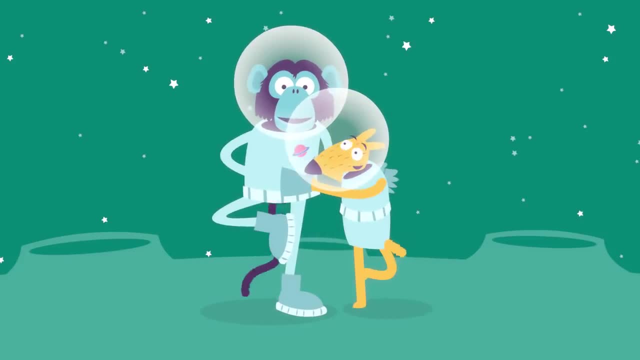 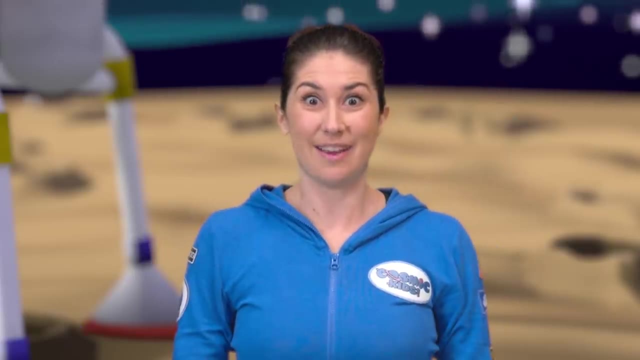 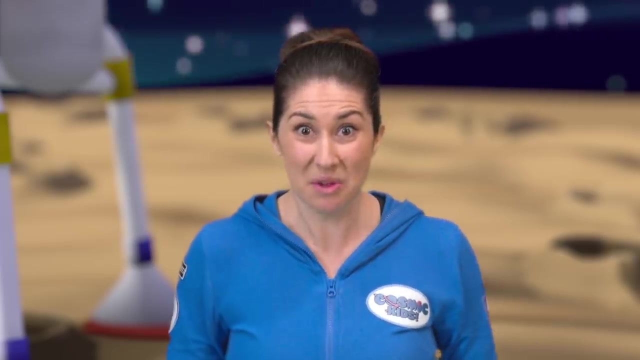 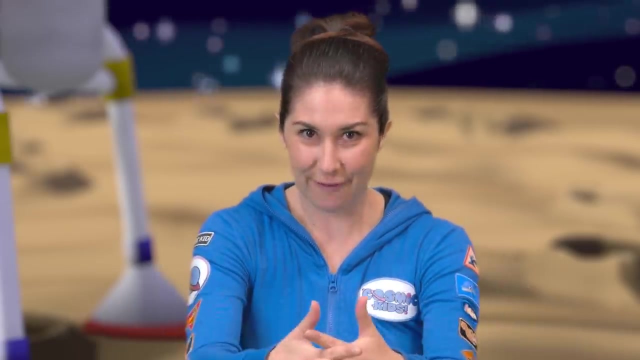 dog. What are Mike and Mutnick doing? They're doing yoga. They're doing double tree pose. This is so exciting, Mike and Mutnick. they live on the moon, So that means we're going into space, We're going to the moon. This is so much fun. Let's start by taking some big, brave breaths. We crisscross. 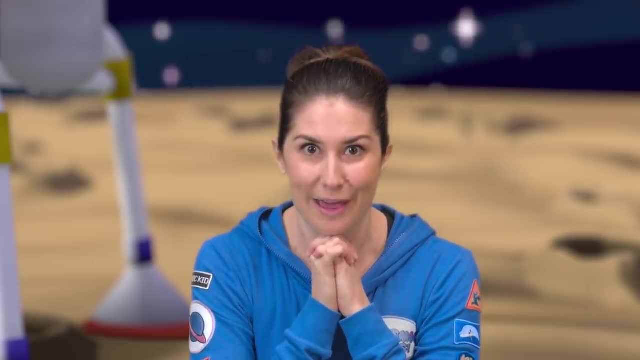 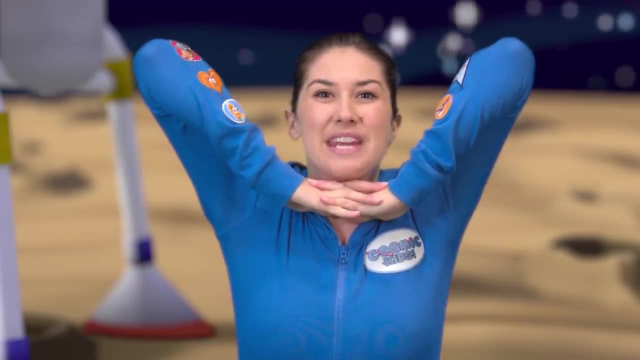 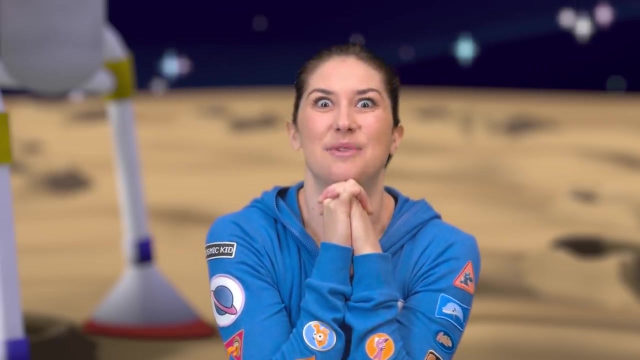 our fingers and put them under our chin and we take a big breath all the way in, Ready, Lifting your elbows high, high, high. And then we breathe up to the sky. Ready, Let's do another one of them: Breathing in, lifting your elbows And breathing out to. 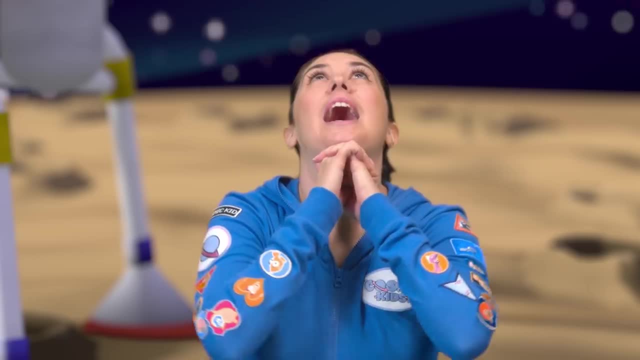 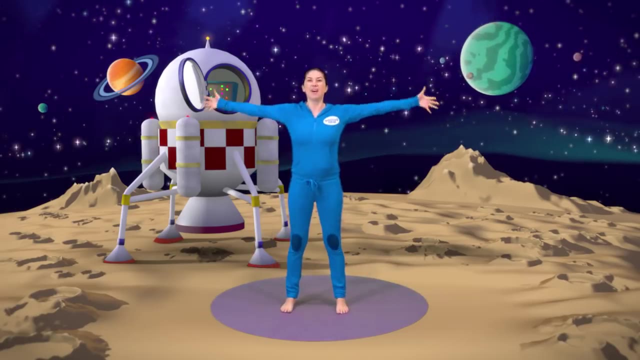 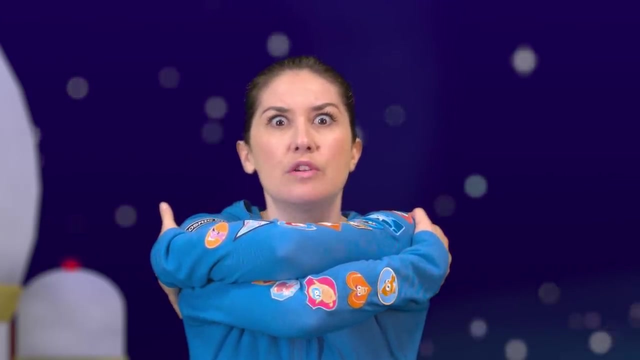 the sky like a dragon. Very good, everyone, Let's stand up now and take our arms wide to give everyone at home a great big hug. goodbye, Bye, everybody. And out of the corner of our eye, we spot outside in the garden. 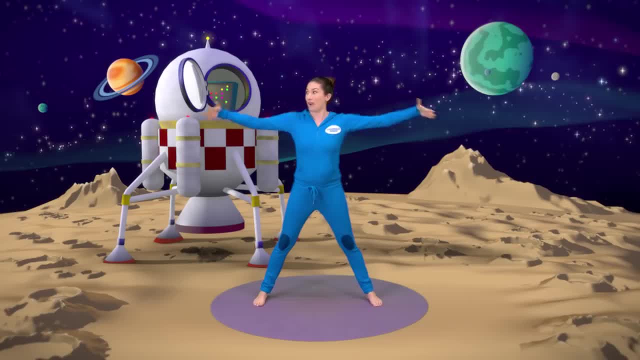 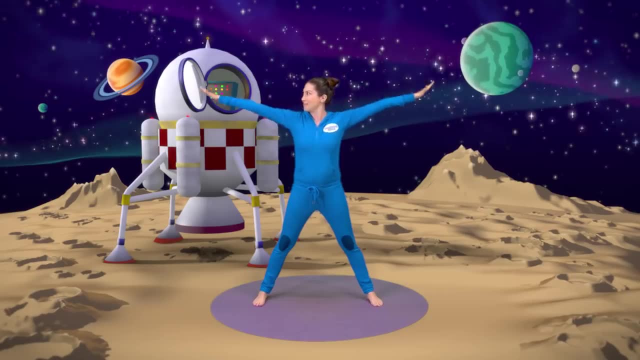 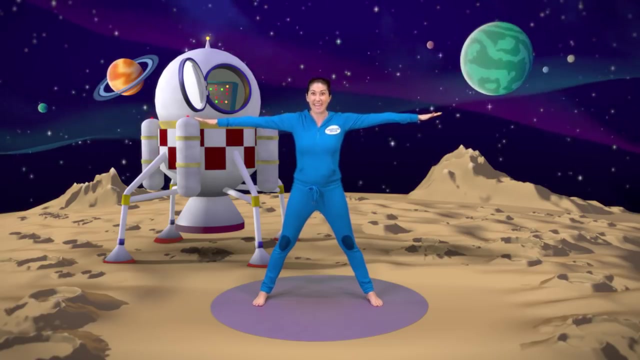 our rocket. Jump your feet wide, take your arms wide and bring your hands above your head. Look at our rocket, everybody, and look, take your arms out to the side. It's got great big giant silver wings. Cool, let's go and get in. We jump our feet together, we squat. 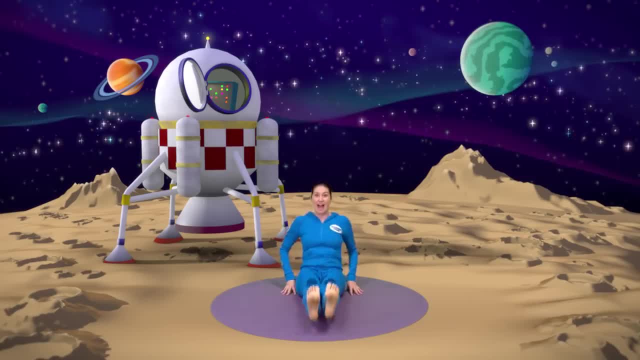 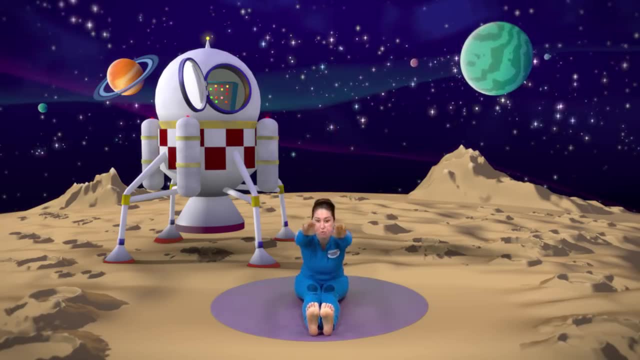 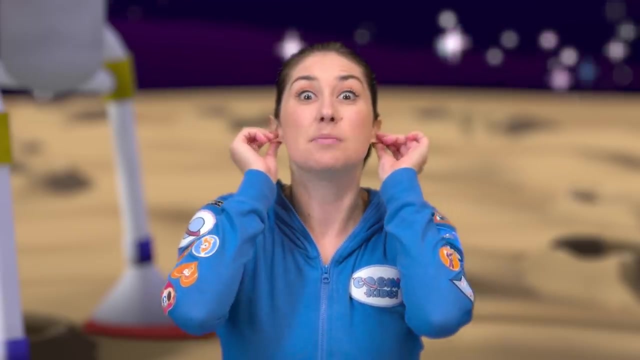 all the way down, and then we sit with our legs out long, We reach up and we close the big glass door on our rocket, Bending our knees a little bit to touch our toes. Now we're in our rocket, we activate our ears by giving them a rub all the way round, so 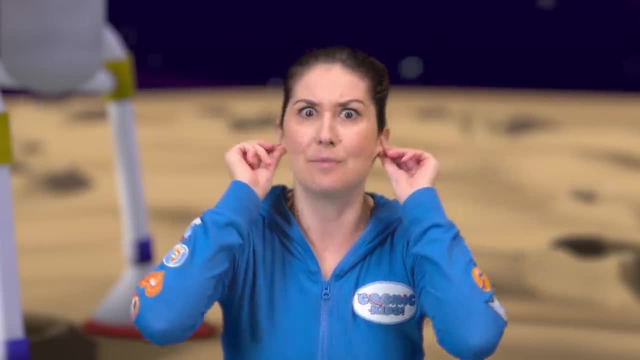 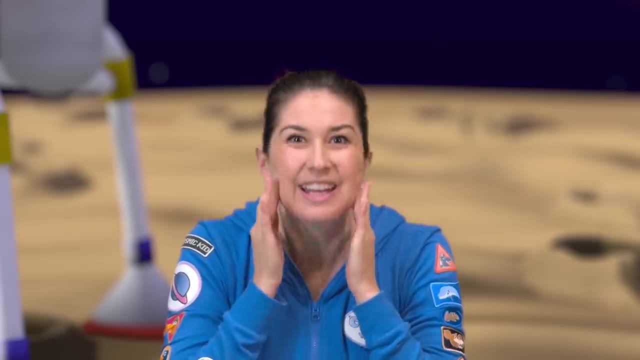 that we can hear important messages. Oh, and we need to activate our voices so we give our jaws a really good rub as well. Well done everyone. that means we can speak too. Now we need to turn our rocket on. So we fold forwards and we turn on our rocket. Now we 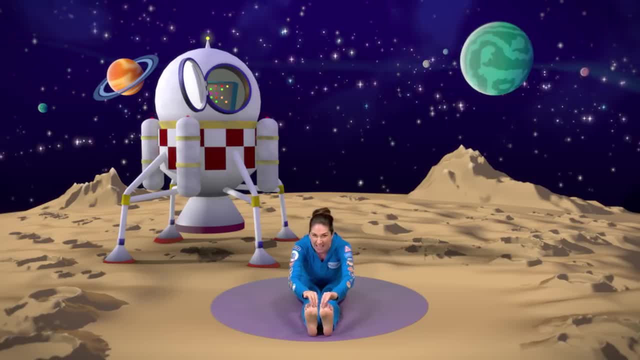 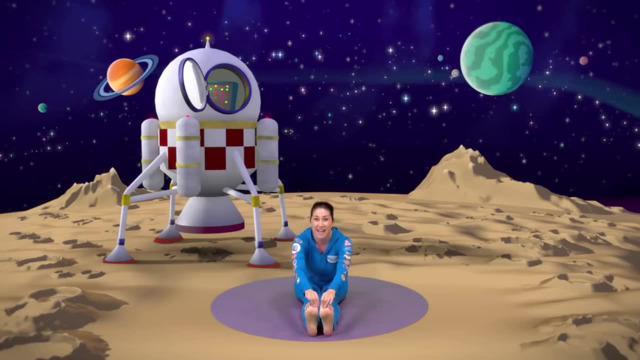 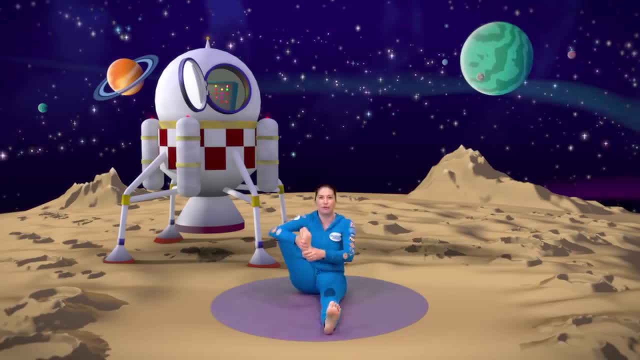 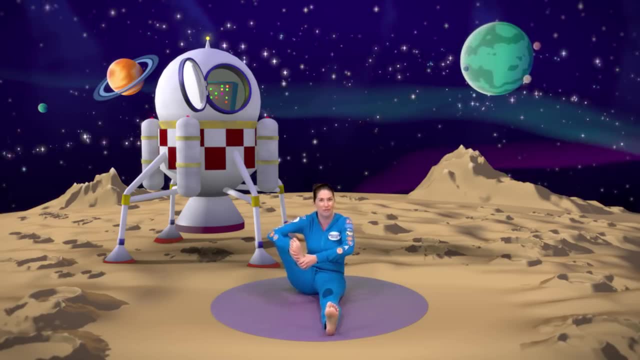 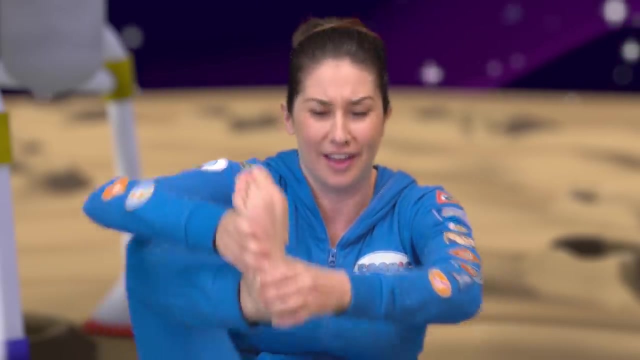 Now we need to check the steering controller's work. Lift up one of your feet and take it over one side And the other, All the way forwards And all the way back. Well, that one works, let's try the other. Putting that one down. 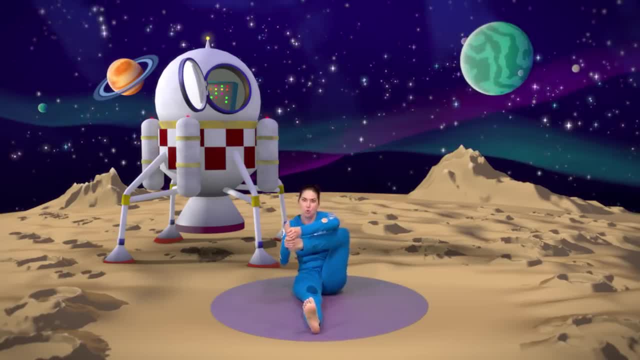 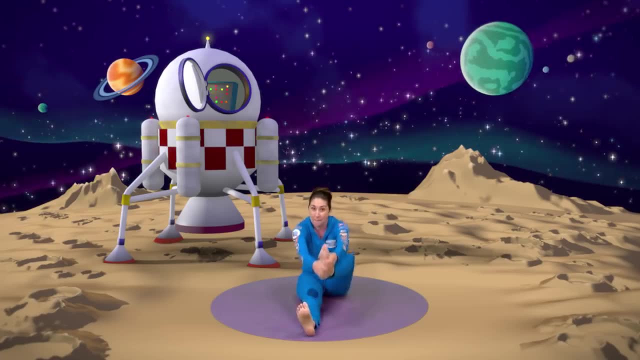 Lifting up the other side. now Ready Beep boop boop. And the other way Beep boop boop. Forwards Beep boop boop And backwards Beep boop boop. That one works too. I think we are. 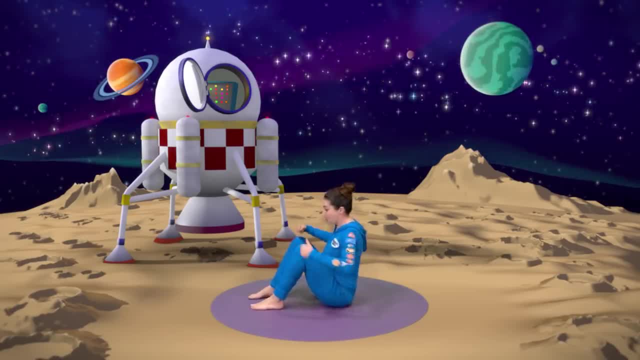 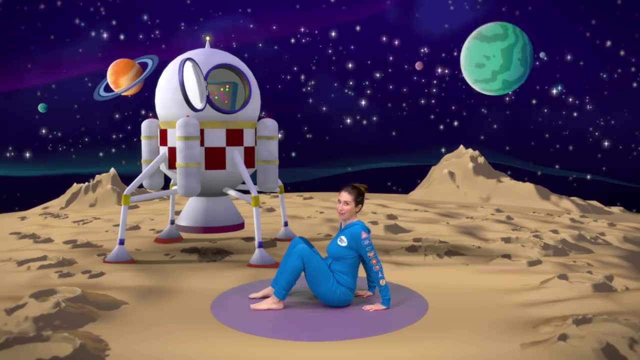 ready for take off. Now, turning to the side, we bend our knees, put our feet flat and take our hands behind us, And as we lift our hips, we count down from five Ready, Here we go. Five, Five, Four. 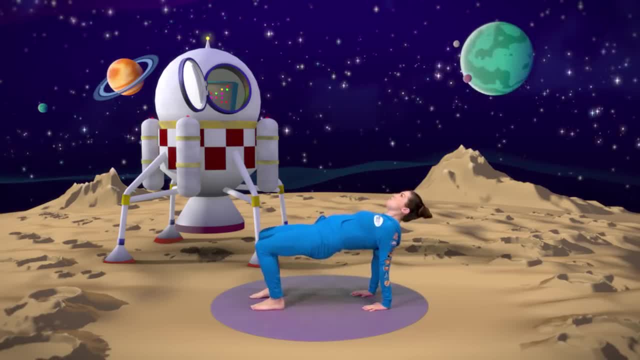 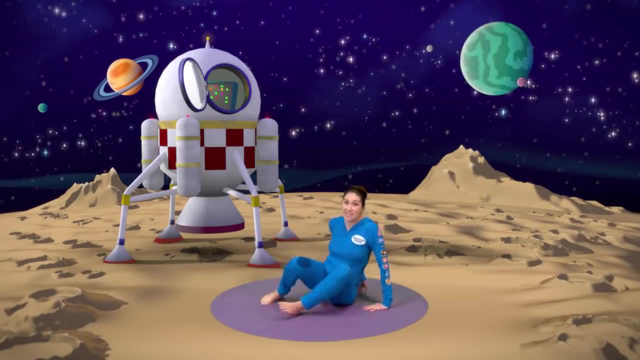 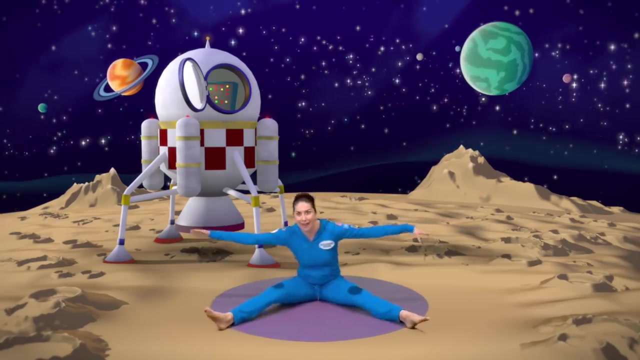 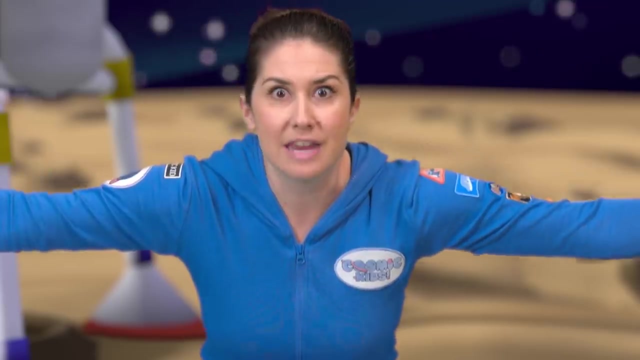 Three, Two, One Fire And blast off. We sit with our legs wide, everyone, as we rumble up into the sky, We go over to one way and over to the other way, And then we break through Earth's atmosphere and we feel. 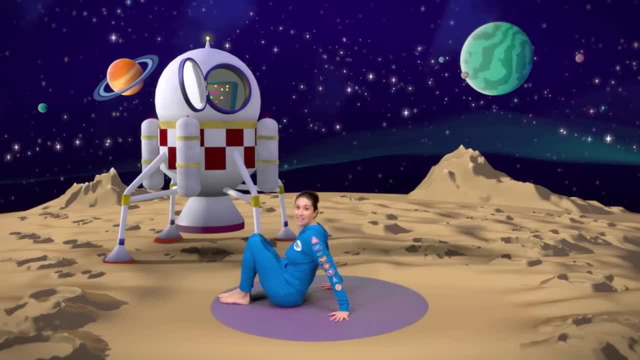 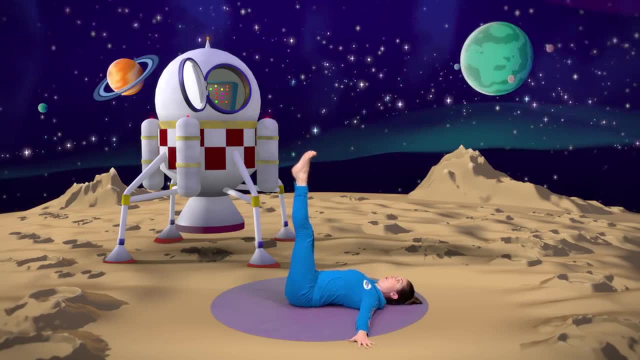 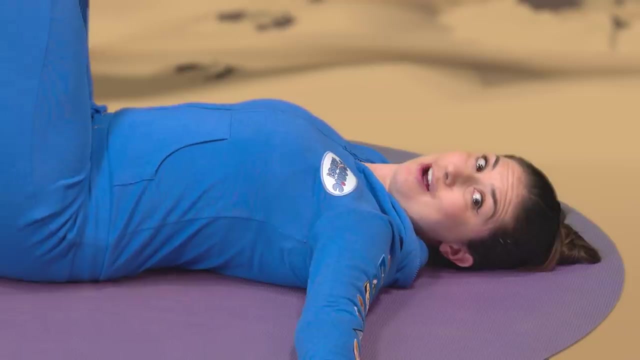 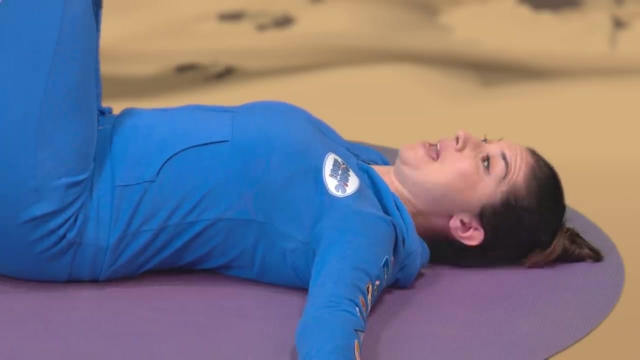 zero gravity. We lie on our backs in our seats with our arms wide and our legs float all the way up. Wow, We're going into space And it's so lovely. Outside our window we can see a gazillion stars. It's so peaceful out here, Amazing. 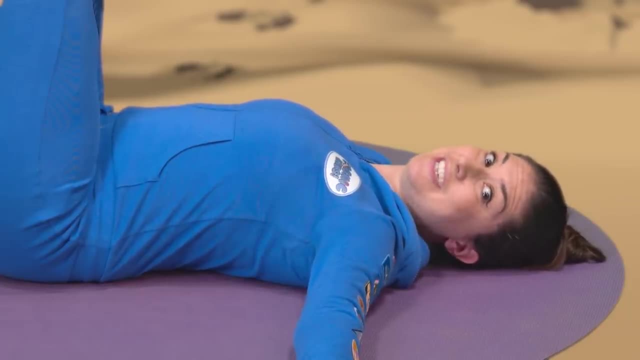 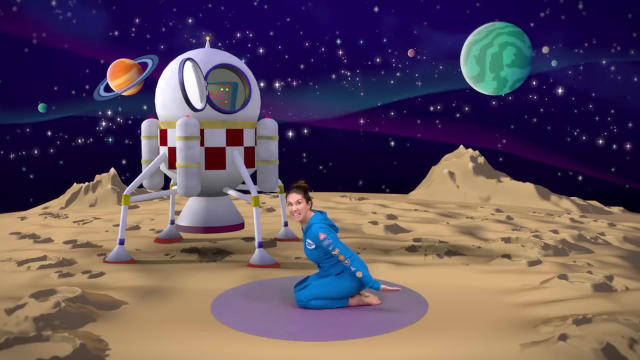 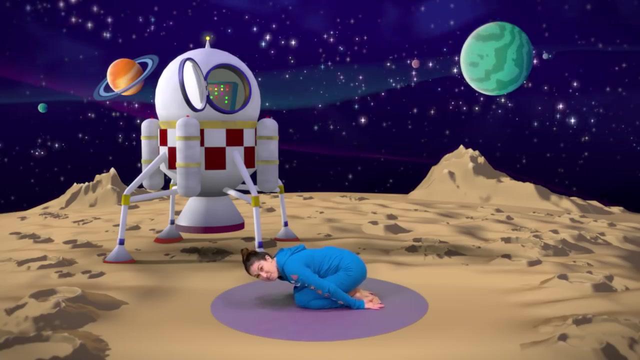 Did you hear that? Yes, It's the landing warning. We need to get into our landing position, Coming up, everybody Onto your knees, Tuck yourself up into a tiny little landing ball. We've landed on the moon. Let's wiggle forwards onto our bellies and have a look through our 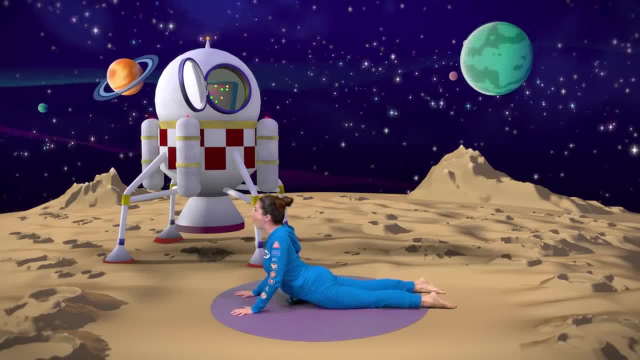 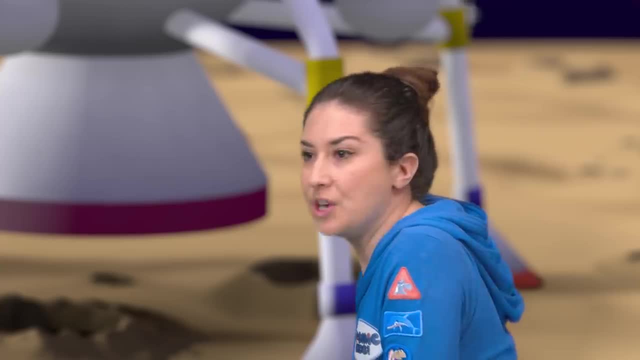 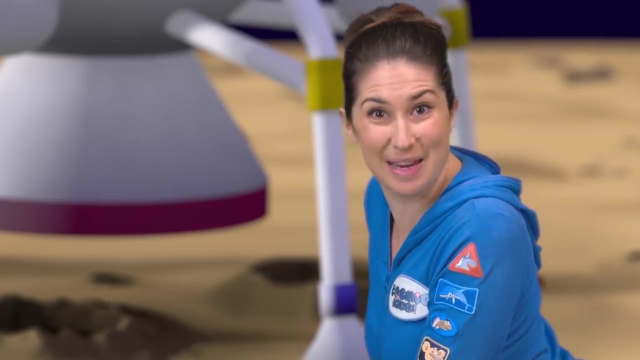 little round window: Wiggle, wiggle, wiggle. Oh, Look out there, everybody, It's the moon. We check our wings are okay. Look into each side, Yep, And looking forward, we can see Mike, the cosmic space monkey. Let's get into our space suits Coming up to stand everyone. 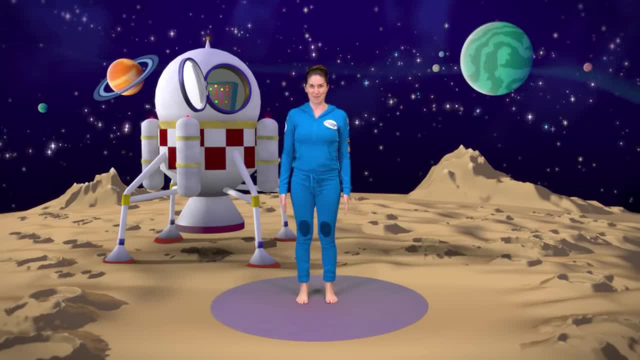 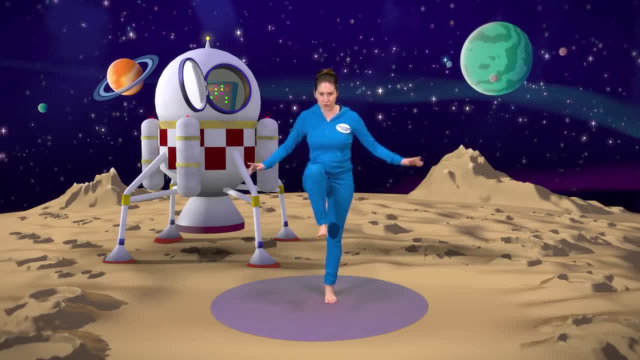 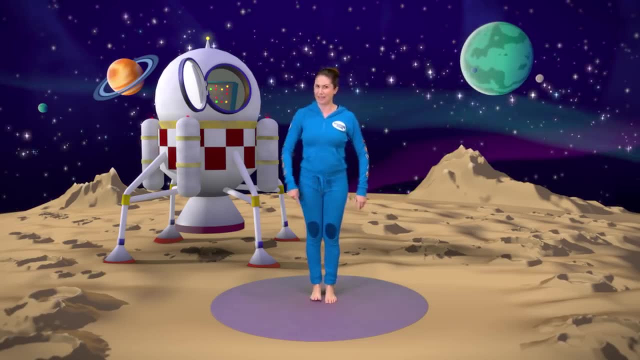 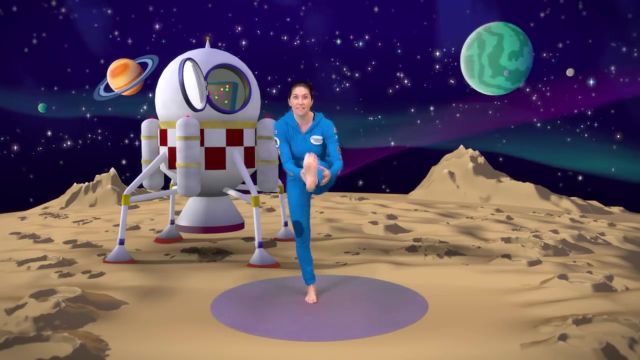 We need to put on our jet pack moon boots. We lift up one foot- Oh, Try not to wobble- And we put our boot onto our foot. Very good, everyone, Let's try the other side now, Lifting up the other foot, Holding onto our moon boot and pop it on. Very good, Now our helmets. 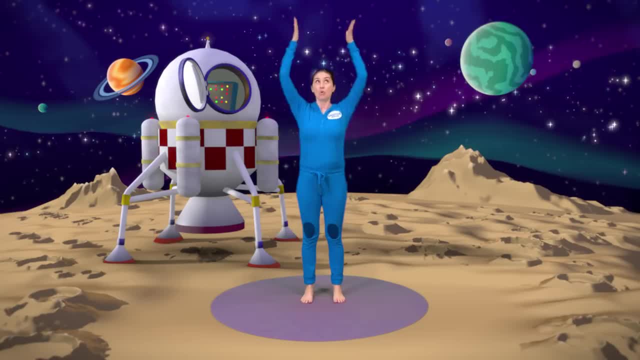 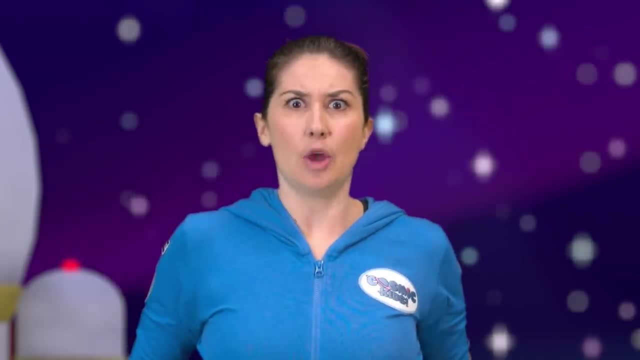 We reach up for our helmet and we put it on our head, Making sure it's secure at the neck, and all of our oxygen works Very good, And now we need to open up the door. We reach forwards and we lift it up, opening the big. 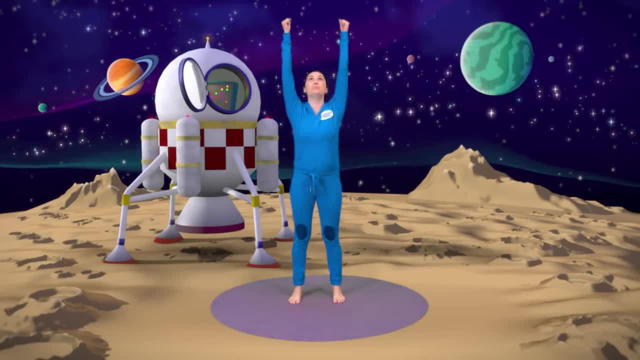 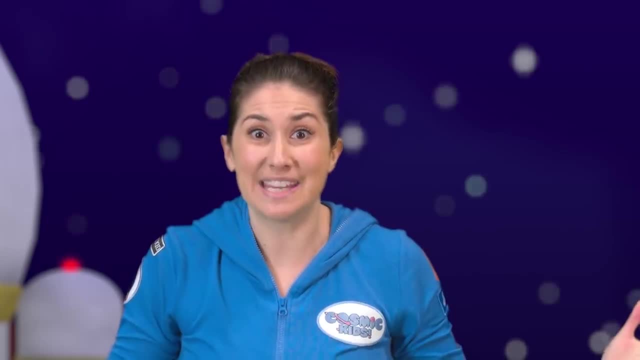 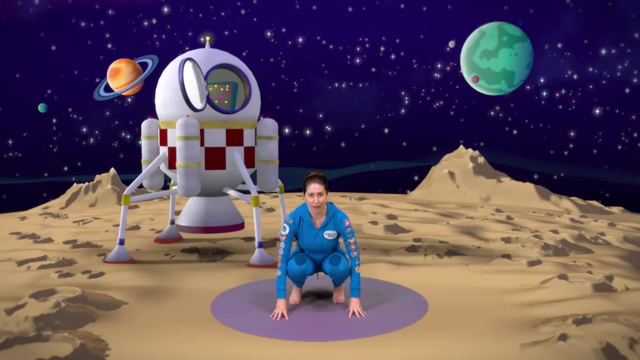 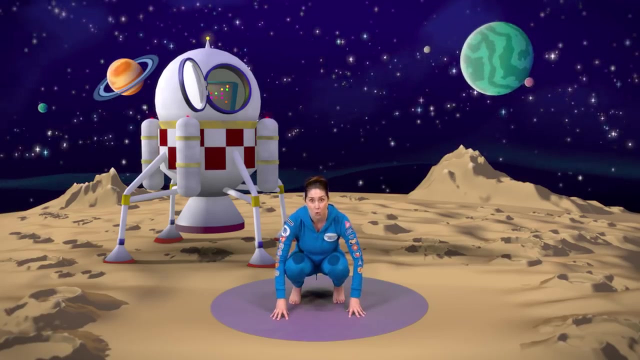 glass door. We say hello space, Hello space. And Mike, the cosmic space monkey, is here and he does a big anti-gravity monkey jump, Now coming down to crouch. It's quite hard doing a monkey jump in anti-gravity because it happens very, very slowly. 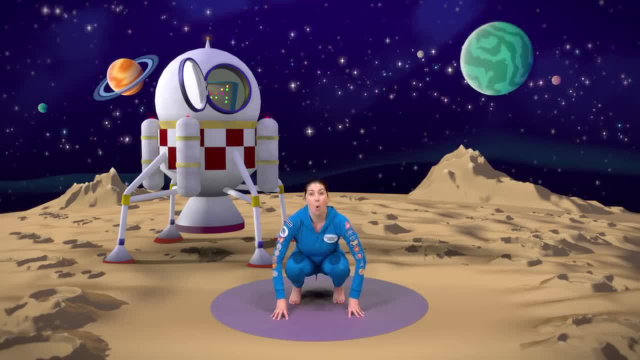 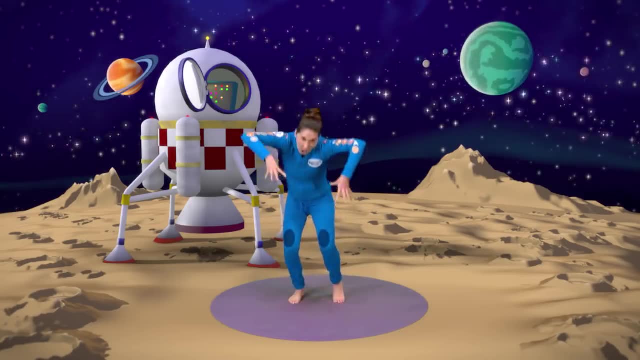 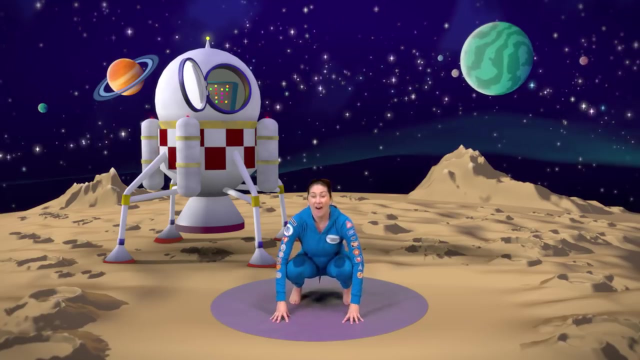 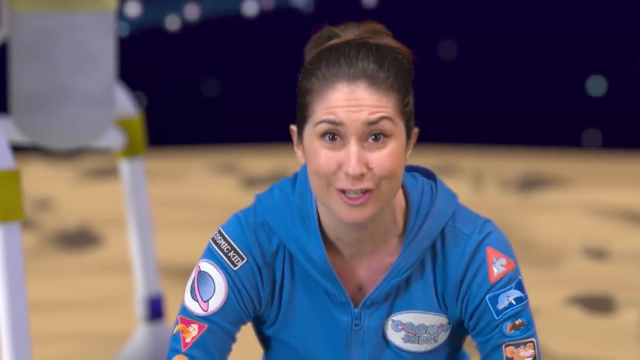 Ready After three. One, two, three. Oh Mike, the cosmic space monkey. Oh, I'm so pleased to see you. It's great that you've come all this way. You're such good friends. But I need your help. My astro dog Mutnick. 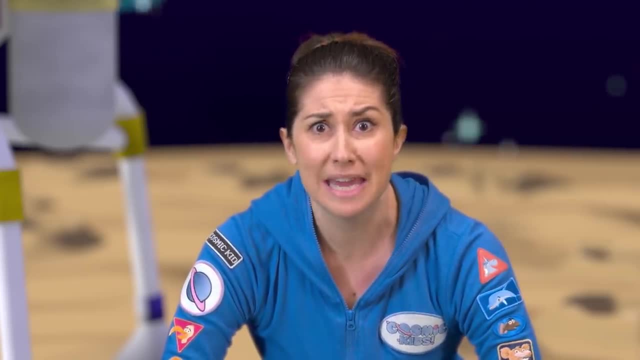 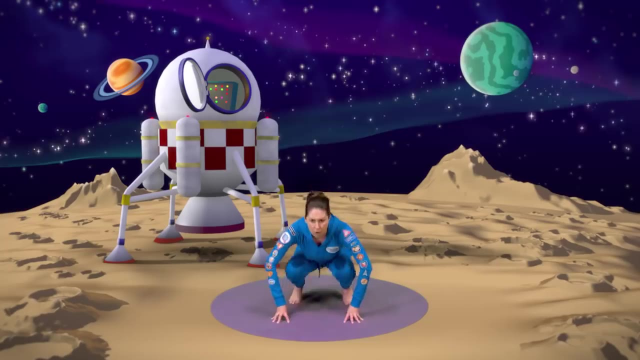 he's my best friend. He seems to have disappeared. I can't find him. Last time I saw him was this morning at the Milky Way Cafe. Do you think you can help me? We stand up. Well, good friends always do look out for each other. I think we can help Mike. 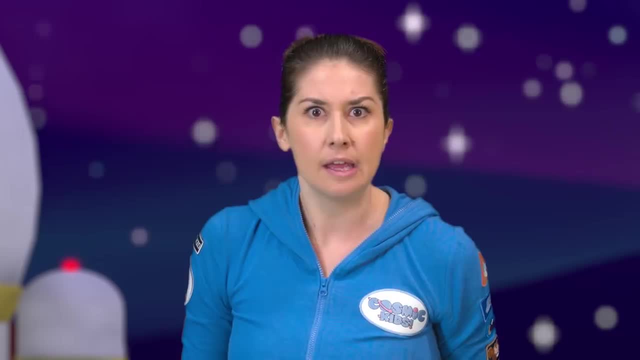 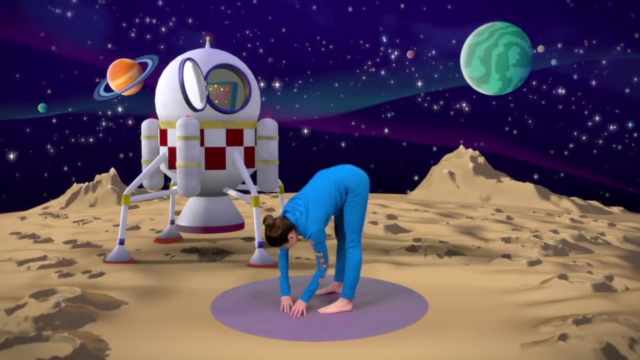 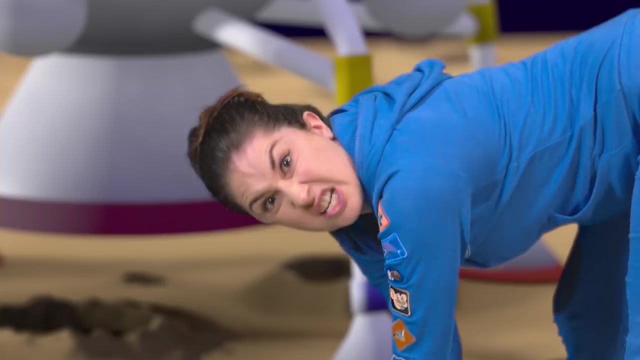 find Mutnick. Hey, did you see that? In the moon dust? Look, folding all the way forwards, We can see something. Use your fingers to clear the moon dust. It's a footprint of a cybersaur. That's a space dinosaur. And stand up everyone, because 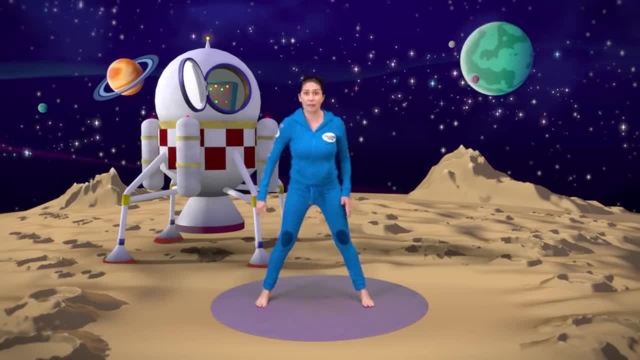 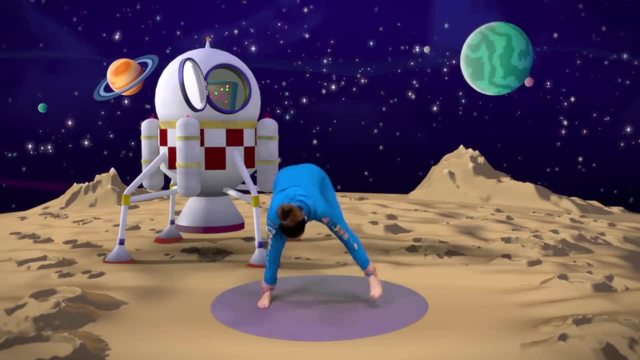 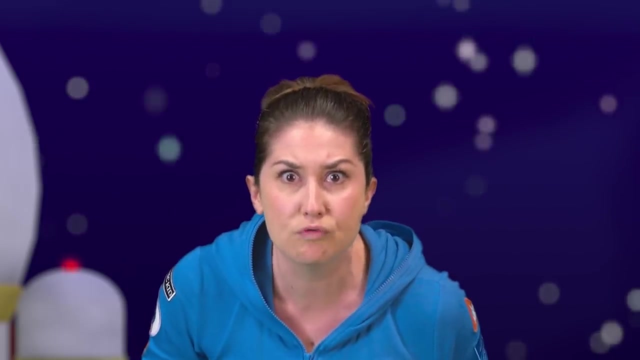 we can hear it coming this way, Turning to the front legs wide fold forwards and hold onto your ankles. He's clumping this way: Clump, clump, clump, clump, clump, clump, Quick everyone. We need to hide behind the moon rock and so he won't see us. 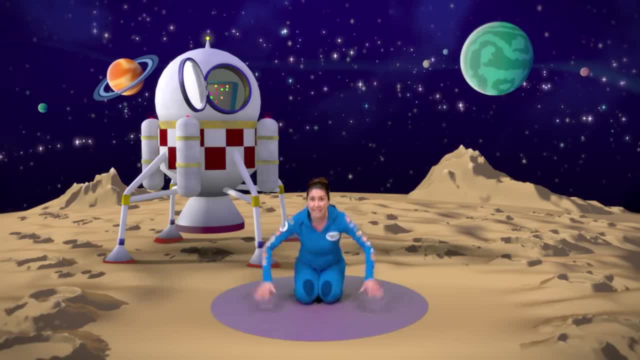 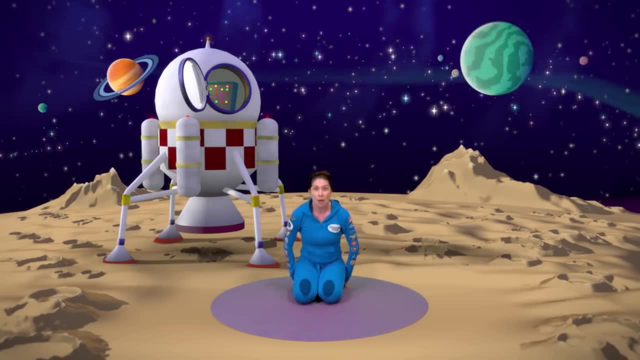 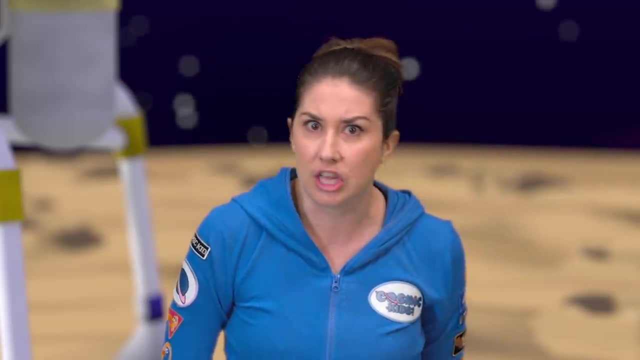 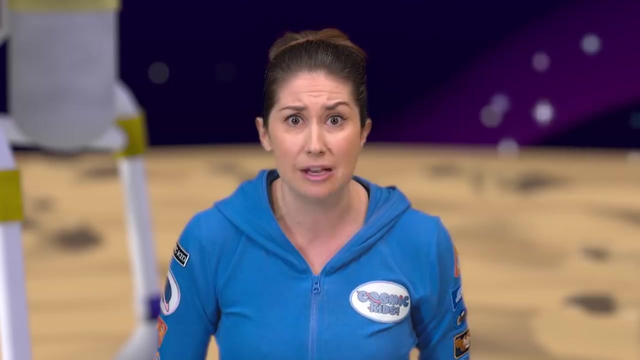 Tuck yourself down into a tiny little moon rock shape. We sit up after he's gone past and we say, Phew Gosh, that's a relief, We're glad he's gone. Maybe Mutnick was running away from the cybersaur and he got a bit lost. Hmm, Let's look through our cosmonoculars again and see if we can. 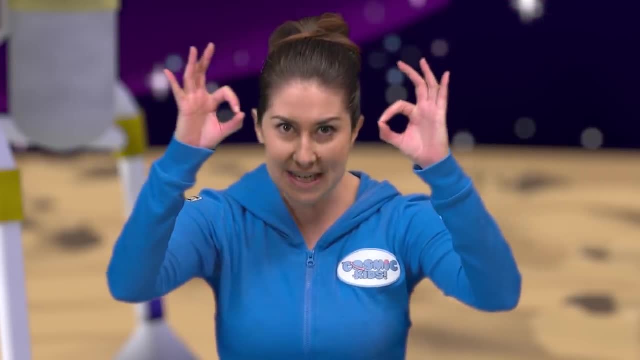 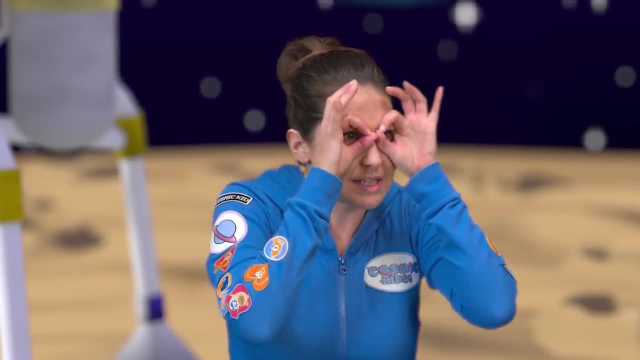 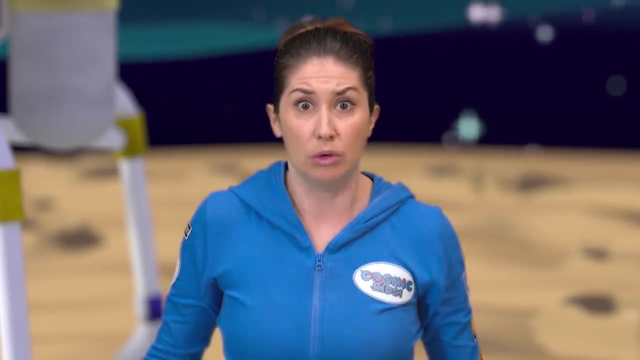 find him Joining your thumbs and fingers together. have a look through. Oh well, it's quite hard to see anything because right in front of us we seem to be looking at the sea of clouds. Oh goodness me, It's quite hard to see where you're going in the sea of clouds. For this we need a crater skater. 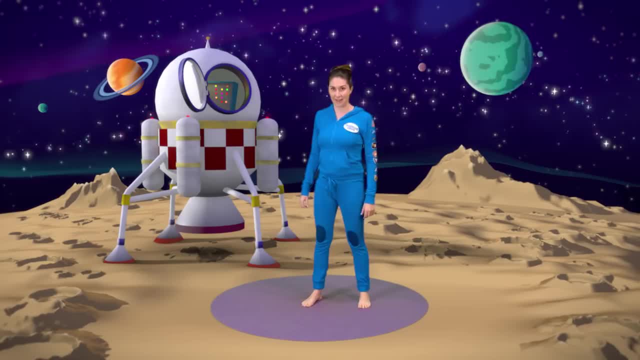 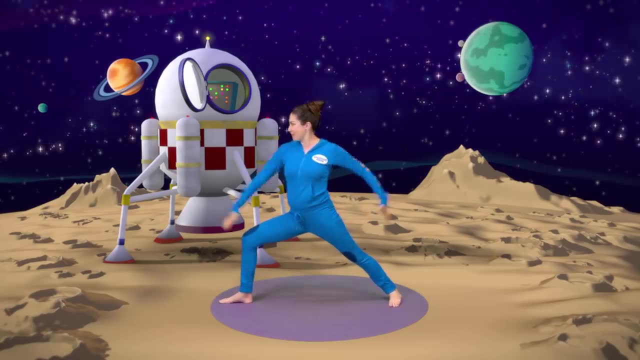 Coming up to stand everyone. We get on board our crater skater so we can be sonic surfers. Put one foot forwards, one foot backwards, Bend your front knee, Take your arms wide and off we go, whooshing across the surface of the moon. 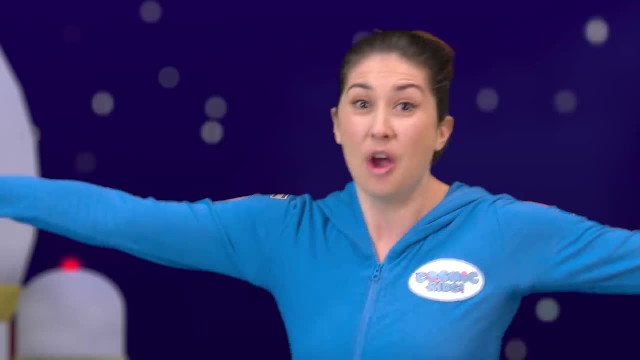 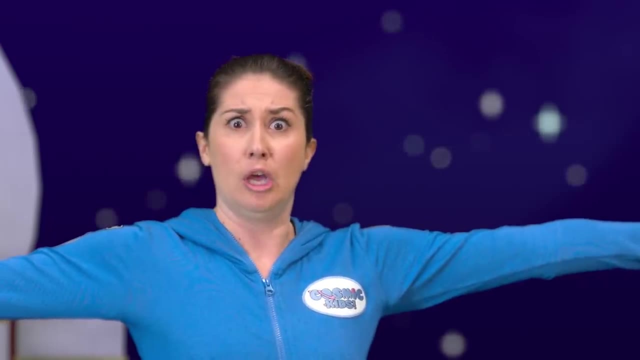 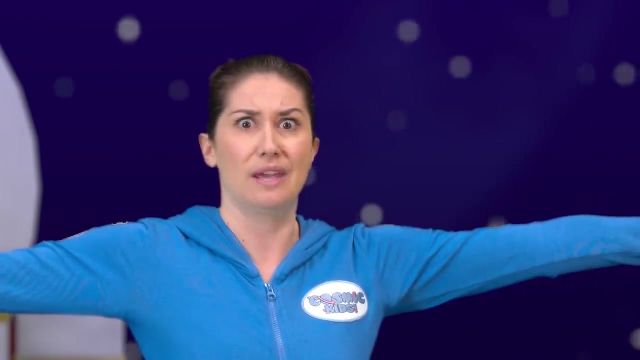 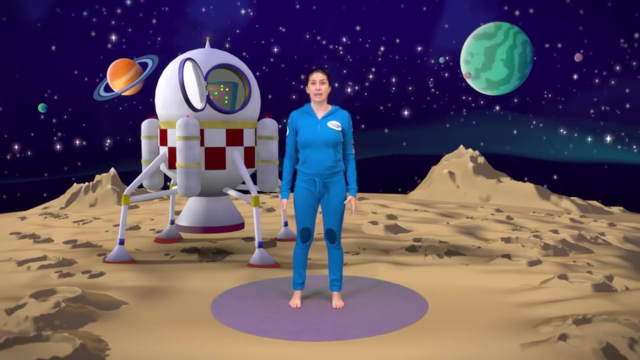 Whoosh, We jump and do it the other way. Whoosh, Uh-oh, We've stopped because we're right in the middle of the sea of clouds and we can't see where we're going. So we stand with Mike like mountains, as still and as powerful as can be, trying to listen with our special listening ears. 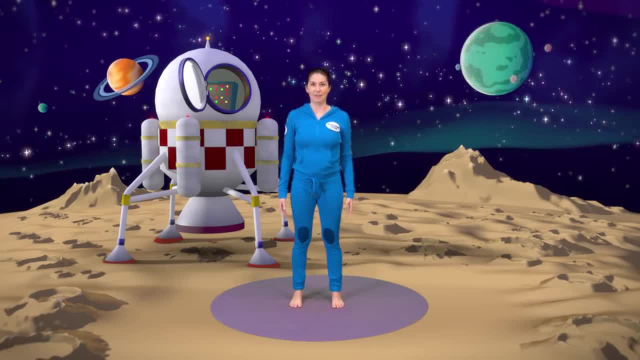 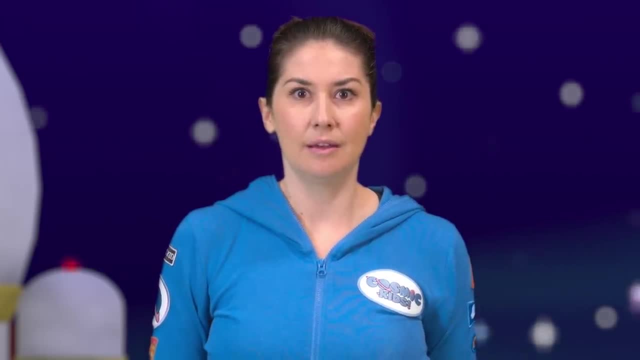 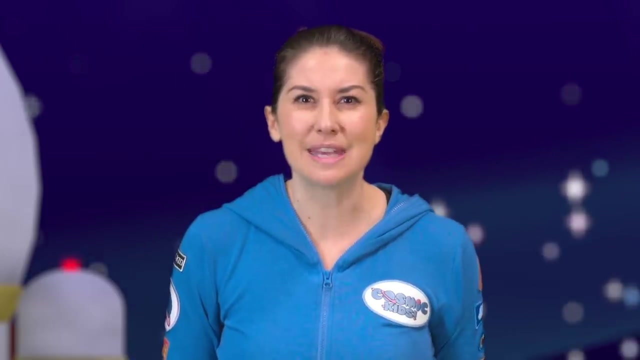 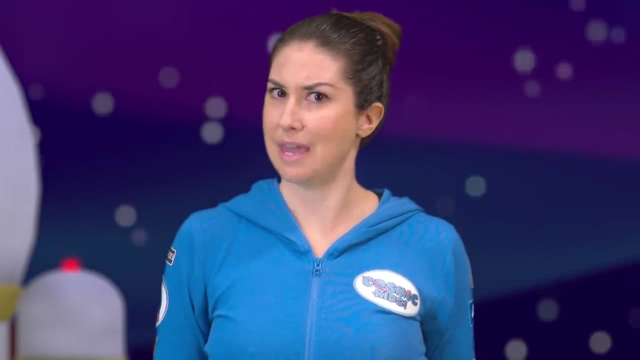 Taking your arms down by your sides and stand very still like a mountain. We hear something: Oowee, Oowee. What's that? Looking with our eyes, we can see through the clouds- A mermaid, Oh, but maybe it's not a mermaid. 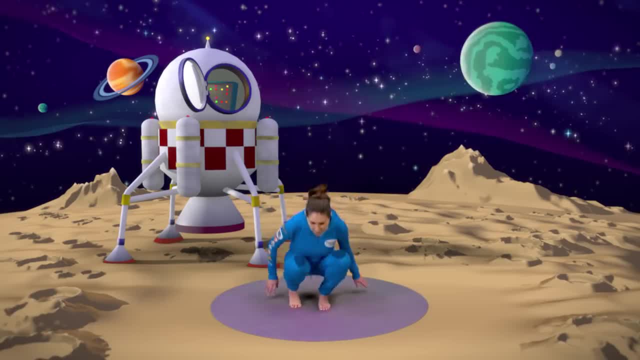 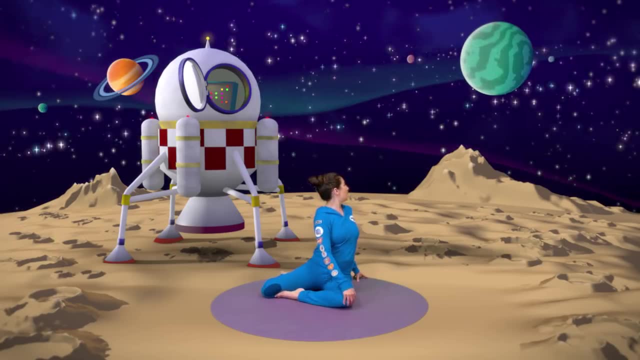 Maybe it's a moon maid Sitting on your bottoms. take your legs around to one side, Put one hand on your knee and the other hand behind you, Looking over your shoulder, then looking to the front. She says it again: Oowee. 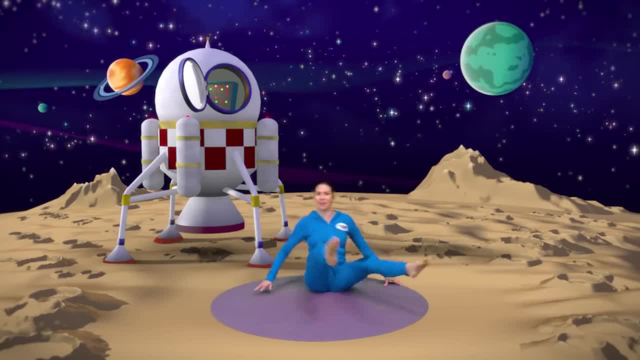 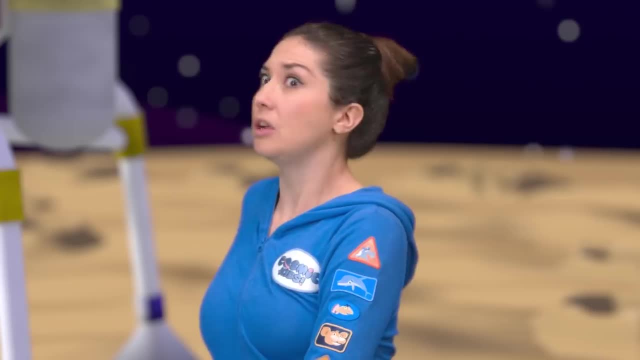 Oowee. Then she seems to swish her tail around to the other side. She puts her other hand on her knee, Her other hand behind her, She looks over her shoulder, She looks back at us and she says Oowee. 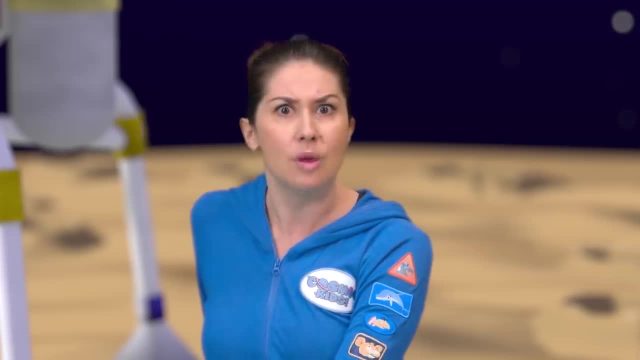 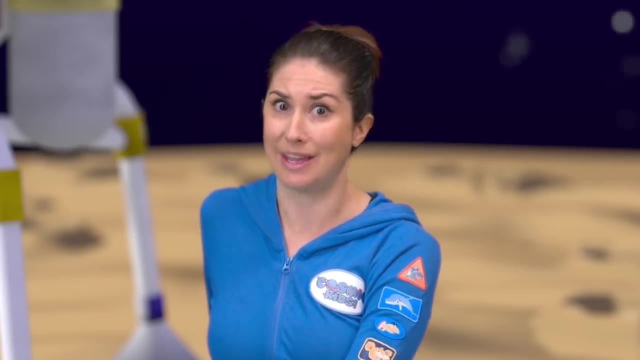 Oowee, She's calling us over. We'd better go and find her Now. to get through the sea of clouds, best thing is to go on our hands and knees so that we can see where we're going. Coming onto your hands and knees, everybody. 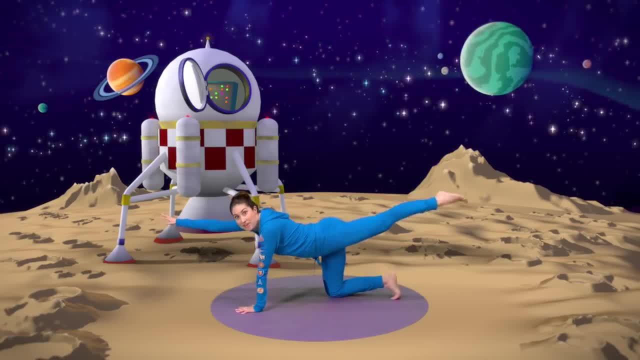 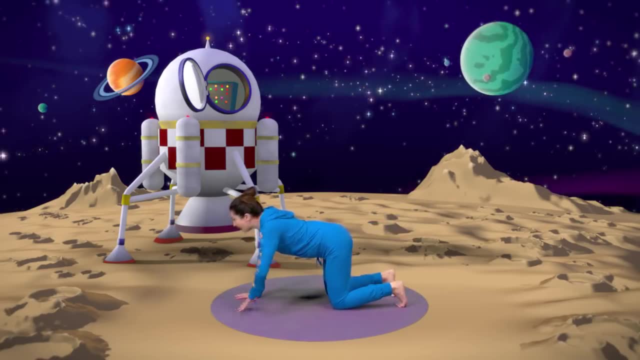 We reach forwards with one arm and reach back with the opposite leg. Oh, well done everyone. We bring that hand and that knee back down and we try it on the other side. Reach with one arm and reach with your opposite leg. Very good, Strong tummies everyone. 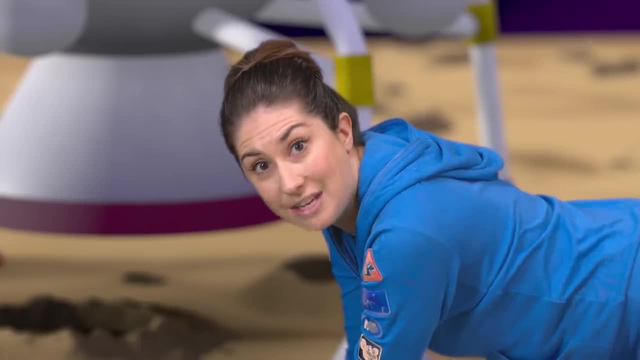 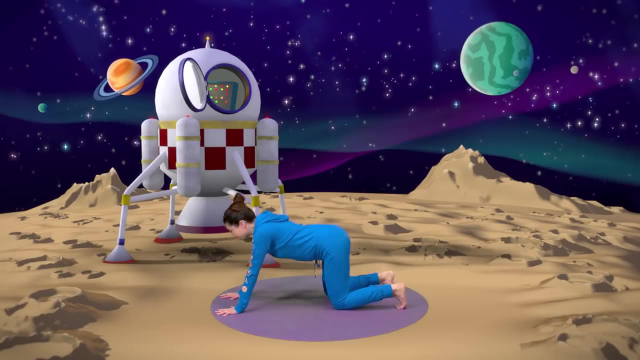 And bring your hand and your knee back down. We make it over to the moon maid, And sat next to her is Matt Nick, the Astro Dog. Hands forward, tuck your toes and lift your bottoms up. He does a happy woof. 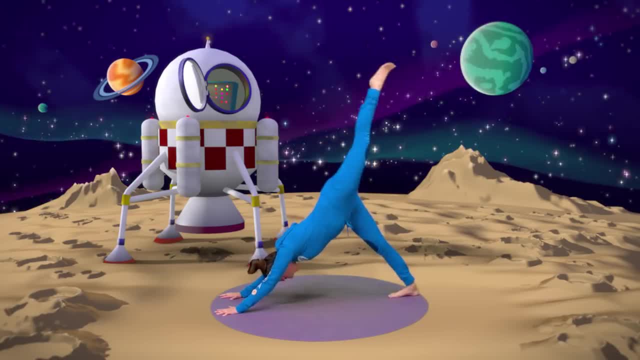 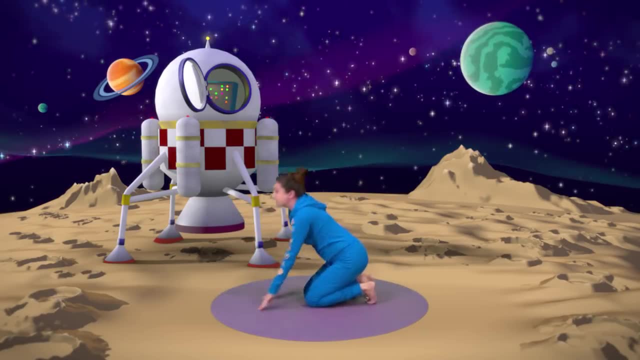 Woof, woof, woof, woof, woof. He lifts up his tail and gives it a good wag. He's so happy to see us Coming all the way down to sit like Matt Nick, with your paws up. 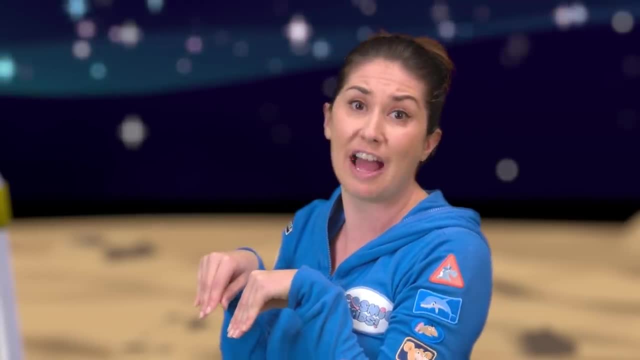 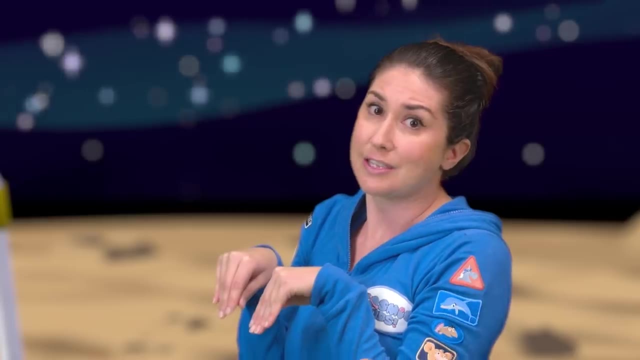 Oh, Mike, the Cosmic Space Monkey, is so happy to have found his best friend, Matt Nick. He's so happy and we're very glad that Matt Nick is safe. It's great that he found help. Whenever you're lost, you should always ask someone for help. 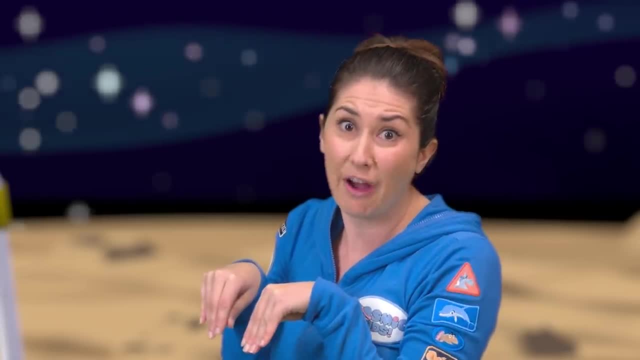 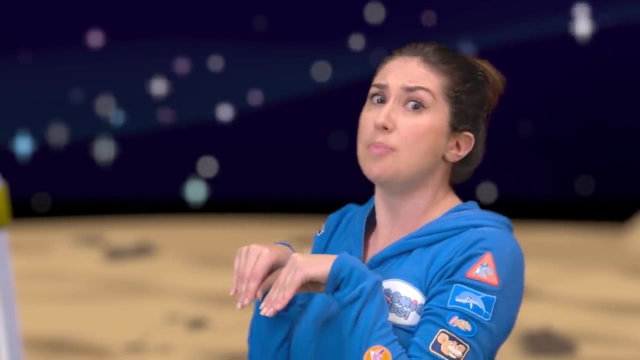 And they will stay with you until your grown up friends come back and find you. Now, Matt Nick is so relieved. Oh, thank goodness. I was running away from the cybersaur And then I ran into the sea of clouds and I couldn't see where I was going. 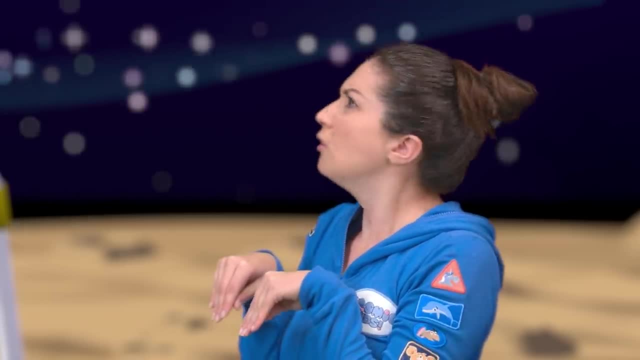 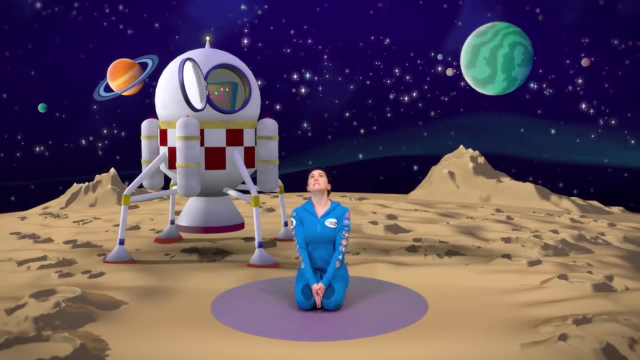 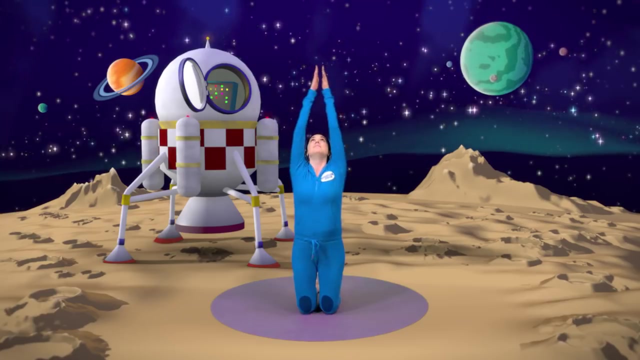 And this moon maid? oh, she's just helped Hang on. Where did she go? We face forwards, We tuck our hands down, We look up And we see the moon maid flying up into the sea of clouds, Breathing in as you lift up. 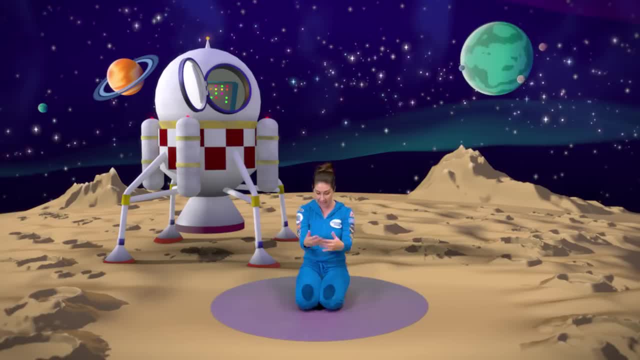 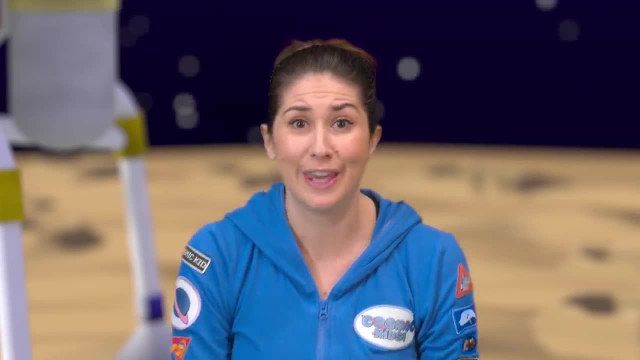 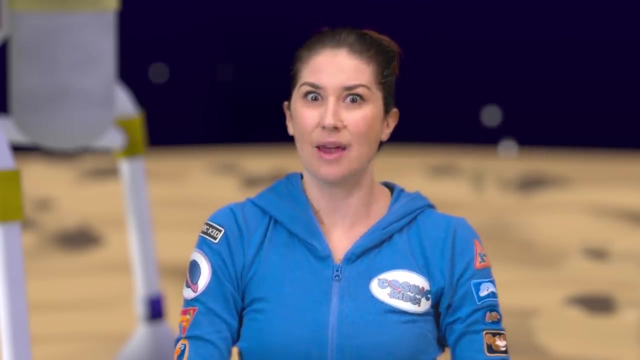 Breathing out as you lower down, Breathing in, Breathing out. We are so grateful to the moon maid for looking after Matt Nick. We blow her a big kiss. Time to get back to our rocket. everybody, We need to activate our jetpack boots. 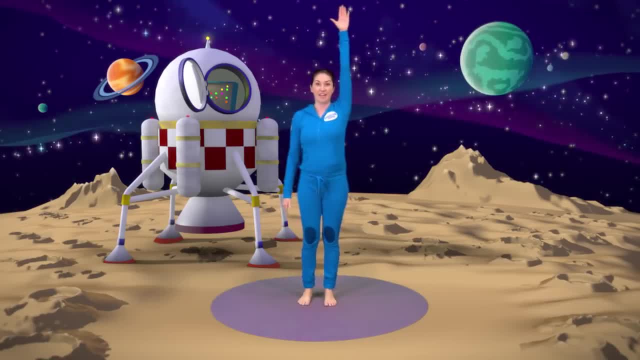 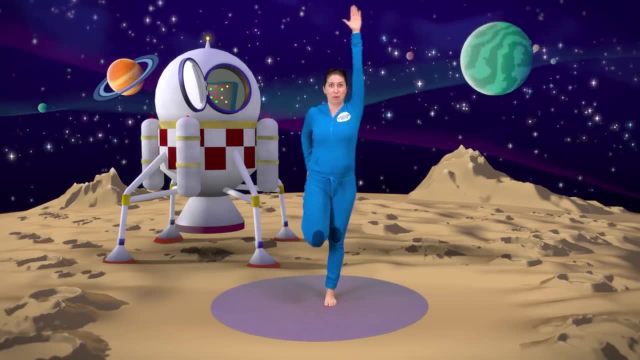 We come up to stand And we reach one arm to the sky, We hold onto our foot And we press the sole of our foot with our thumb to activate our jetpack boots. Try not to wobble. Boop, boop. 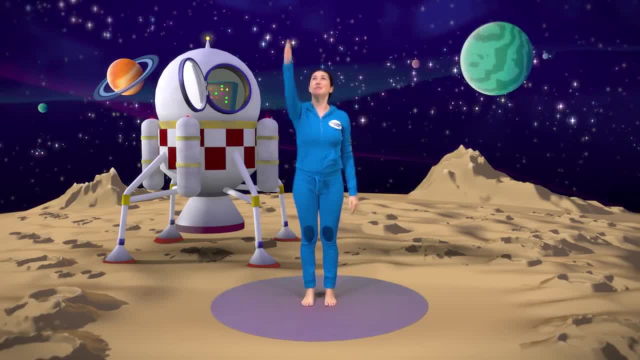 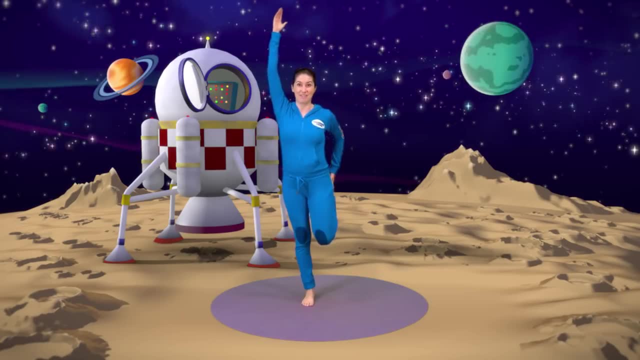 Then we lower that foot. We need to activate the other one. So we lift up our other hand, Hold onto our foot- Oh, try not to wobble- And activate the other. jetpack boot Ready, Boop, boop. 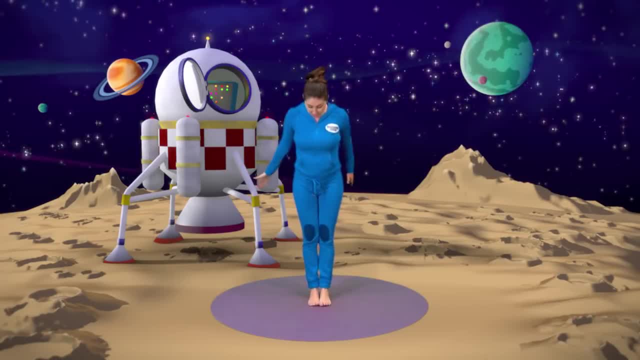 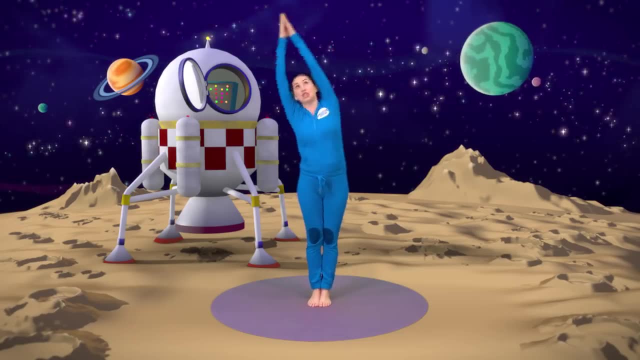 Very good, everyone. We put that foot down, Bring our feet together, Our hands above our head, so we can steer, And off we go Up into the moon's surface, Whoosh, Steering our course all the way back to the moon. 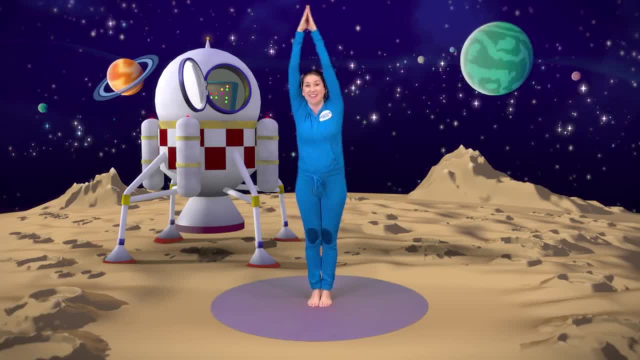 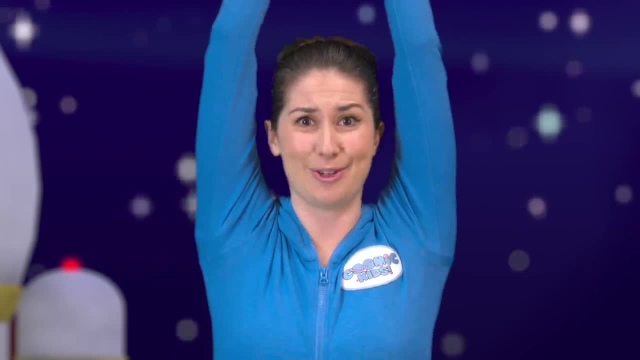 All the way back to our rocket. Well done, Jump your feet wide. We've made it back to our rocket And we managed to find Mutnick the Astro Dog, which is amazing. We give Mike, the Cosmic Space Monkey, a big hug. goodbye. 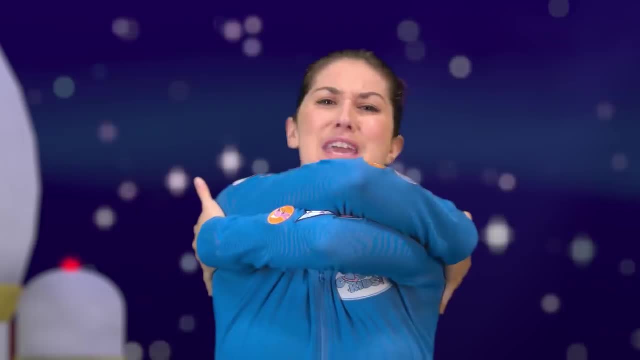 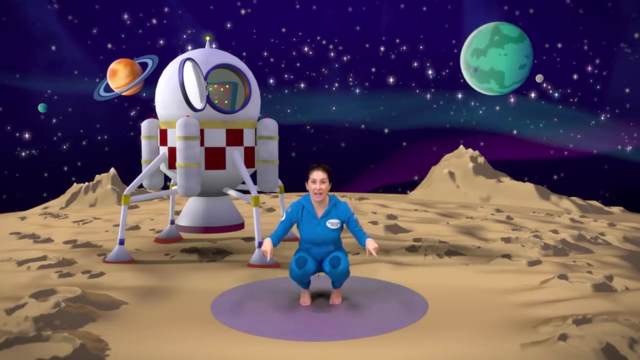 And we open our arms again And we give Mutnick a big hug: goodbye. It's time for us to go home. So we get back into our rocket, Squatting all the way down, Taking our legs out long, Reaching up high. 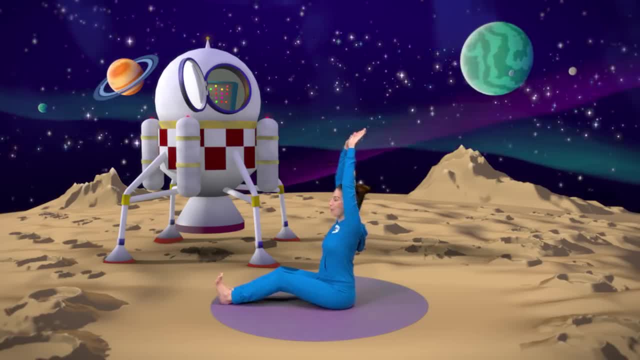 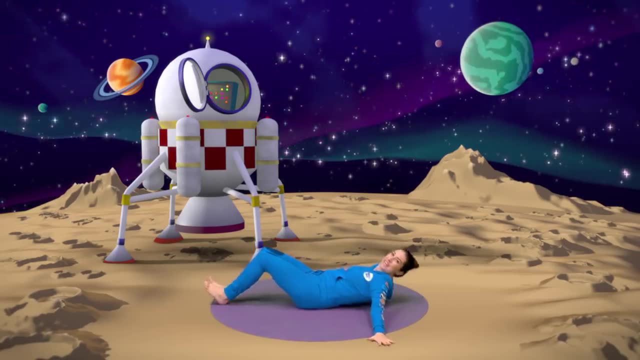 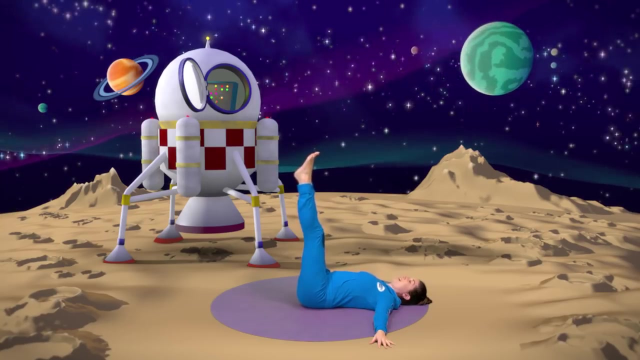 Bending our knees And closing our glass door. Whoosh, Now we lie back And we wait for our takeoff, Taking our arms wide, Our legs up in the air. As we feel that zero gravity once more, And as it's our journey back, we let our legs lower all the way down. 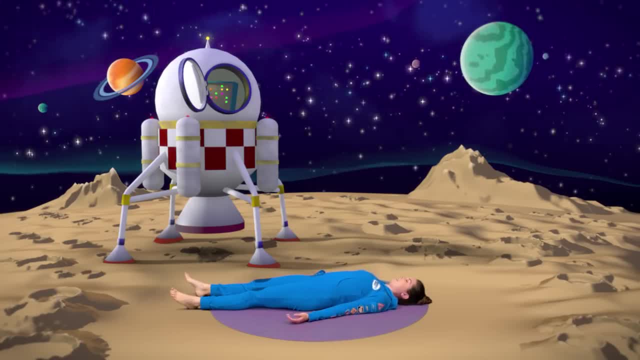 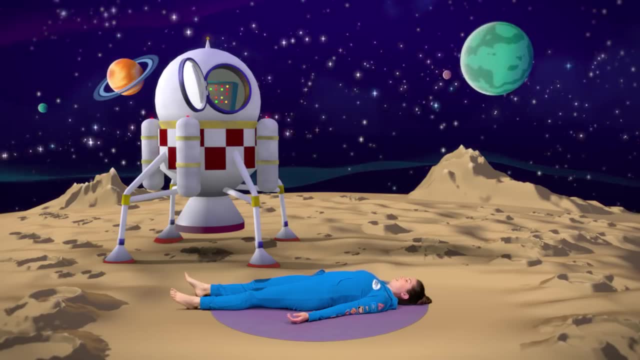 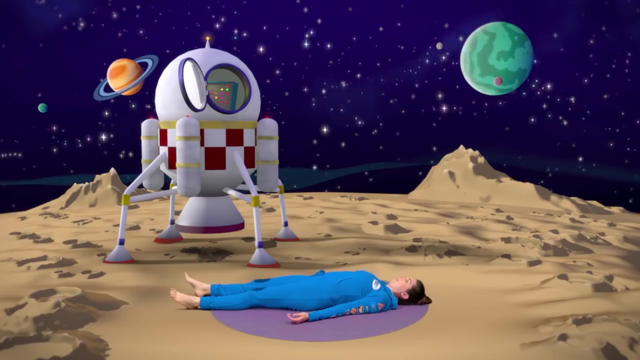 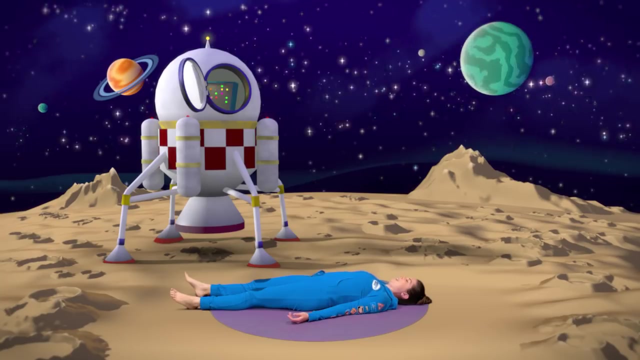 We take our arms down by our sides And we lie back And we rest here in our rocket As it flies through the peace of space. We're so glad that we could go and find Mutnick today, That we could help bring our friend back. 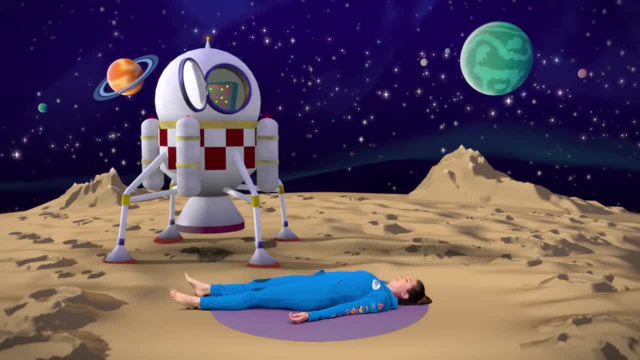 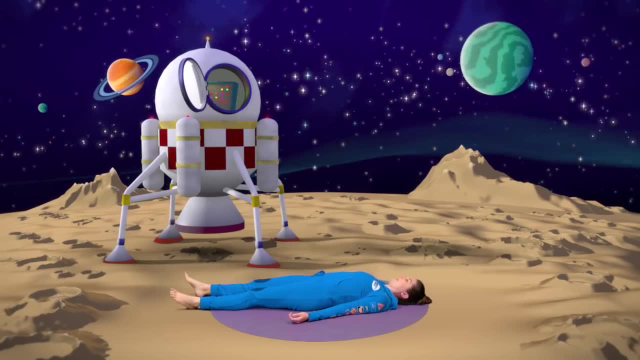 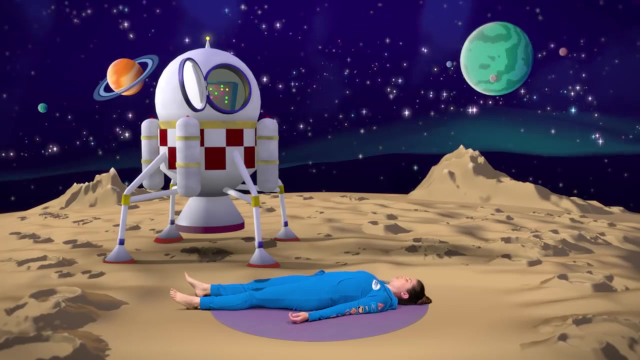 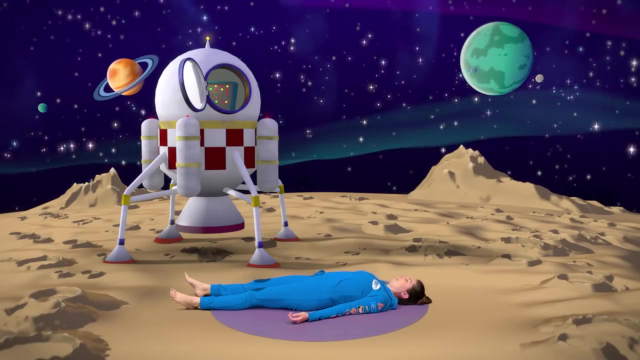 Good friends are so important. You look out for each other, You help each other. You miss each other when you're not there. You look after each and every one of them, Making sure they're safe And doing what they can To always be together. 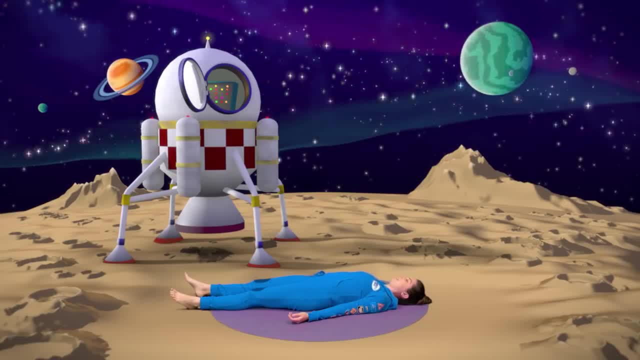 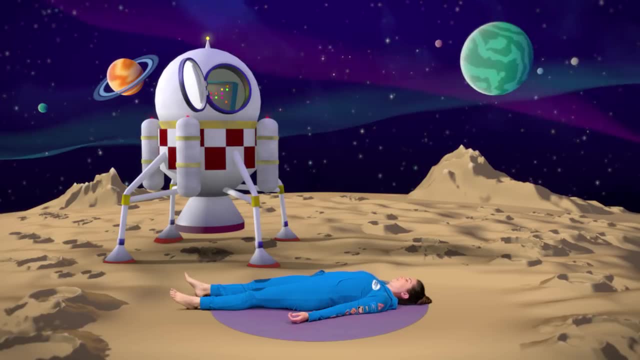 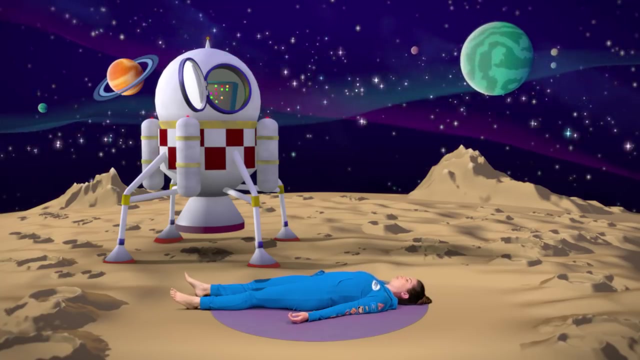 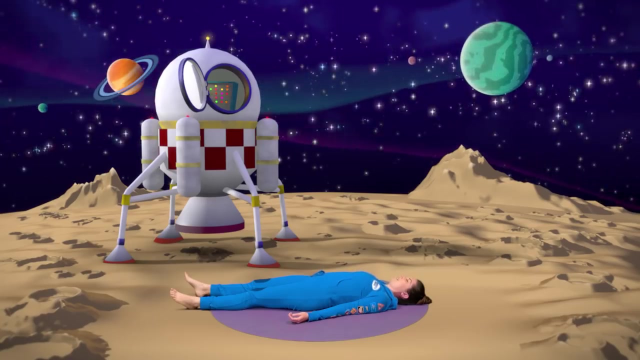 We lie here in this peaceful place And think of our friends, Those people who are special, And we think about what would we do if we got lost, That we would ask for some help From someone who could help us find our grown-up friends. 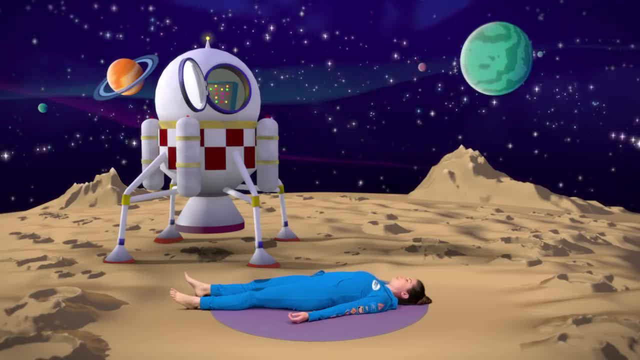 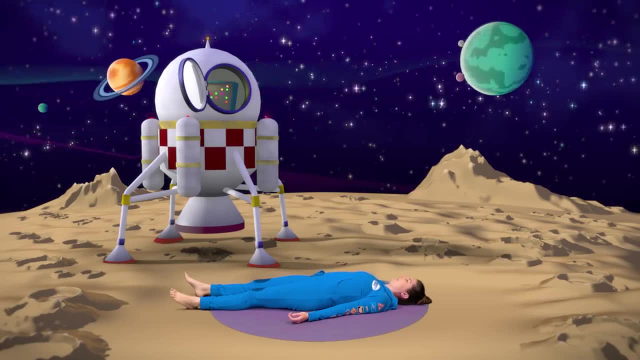 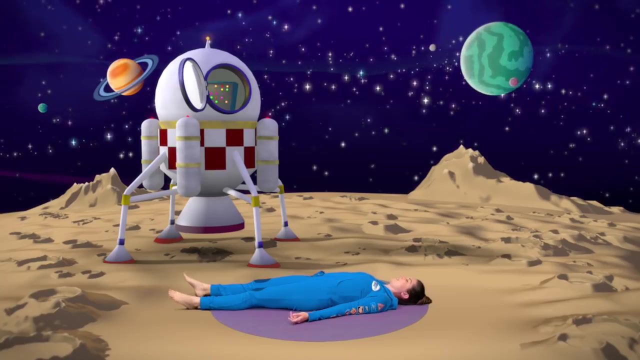 And look after us until they come. That's what Mutnick did. That will mean that we will always be safe, And now it's time to wake up. So we wiggle our fingers and our toes, We hug our knees into our chest. 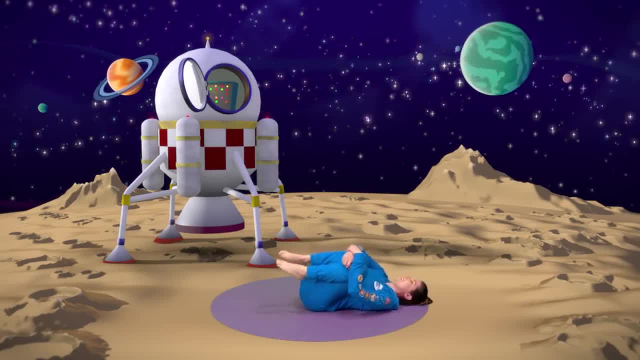 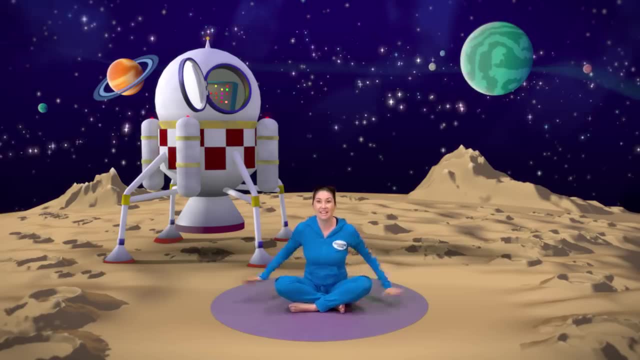 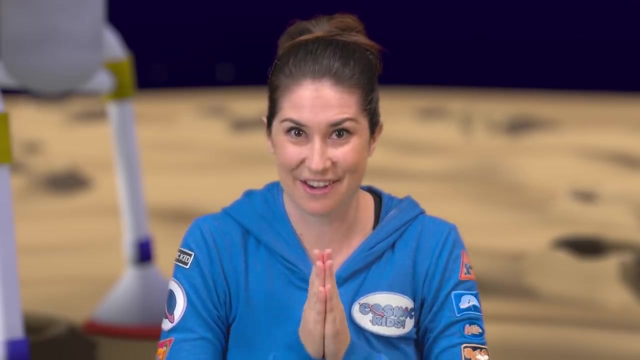 Giving them a big squeeze And we roll over onto our side, Coming up to sit With our eyes open, now Our legs crossed and our hands together at our hearts, And we finish just the way we started With our secret yoga code word.